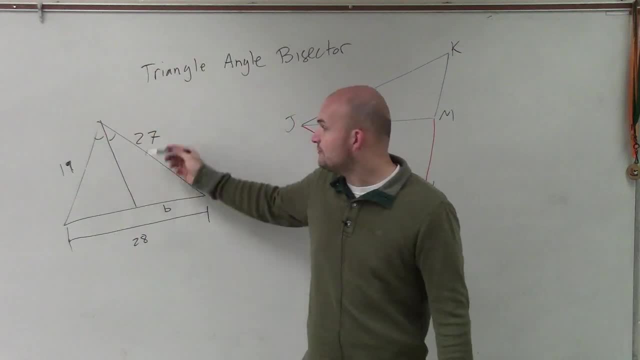 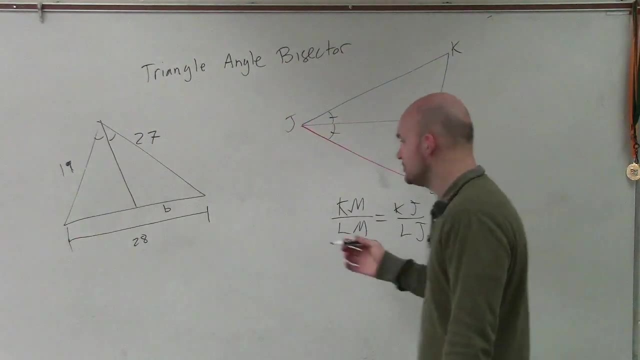 bisector. right, We have an angle bisector, so therefore I can say: would it be okay for me to say 27 is to 19?? Yes, So I'll write one ratio: 27 is to 19.. But now we 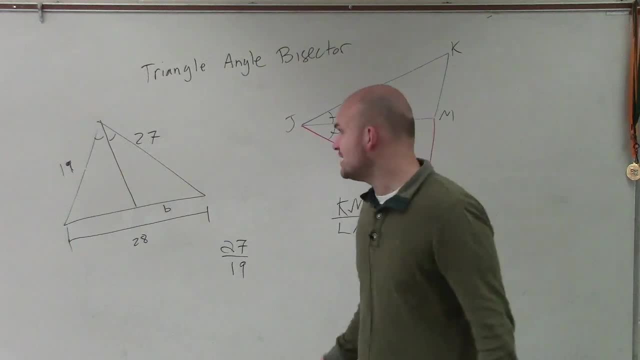 have an issue, because now the problem is: what is my other ratio? What is B proportionate to Well? well, be careful. 28 is this whole segment, Is it half of it, though? Do we know? We know? 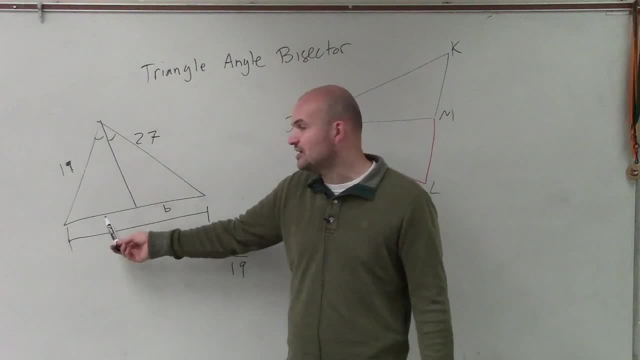 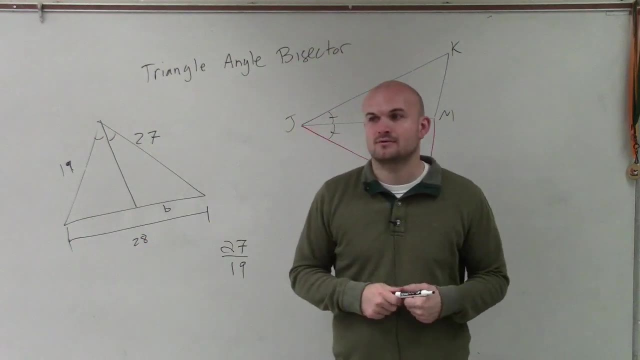 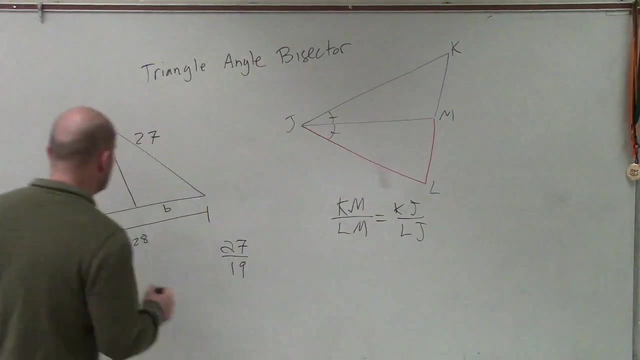 that this line cuts this angle in half, but it doesn't necessarily cut the side in half. So if this is B and this whole thing is 28, what does this have to be? Then you have more variables. yeah, Close, It's going to be 28.. 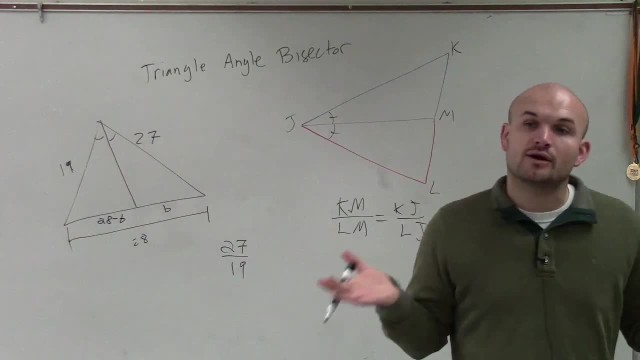 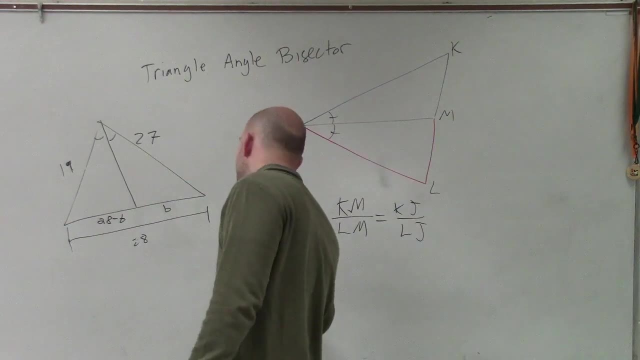 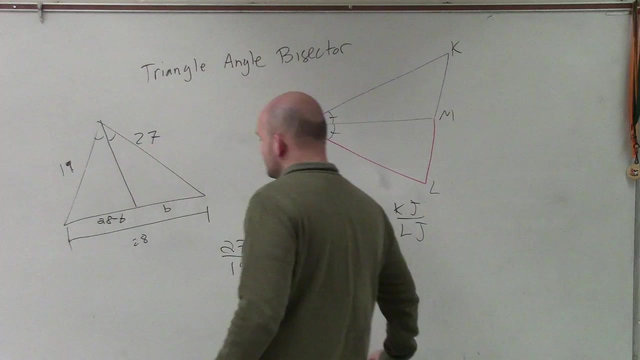 Minus B. Okay, So you're going to want to take the length of the 28 and then subtract B. Now again, we still don't know what B is. However, Malik, now we have a ratio- Oh, I'm sorry, not 28.. But now what we do is we have a ratio that we 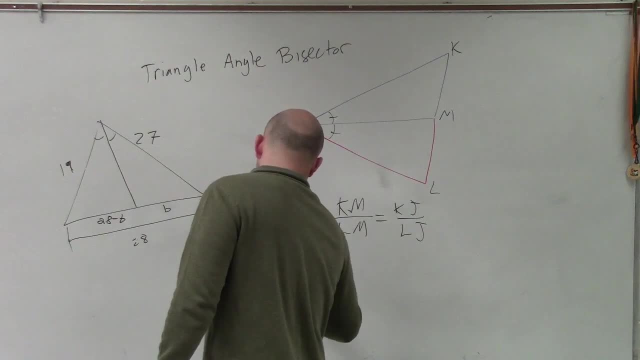 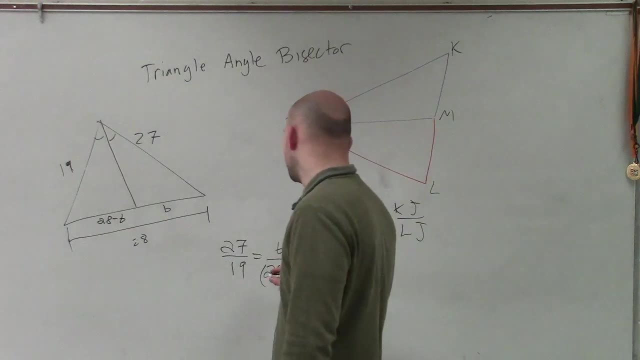 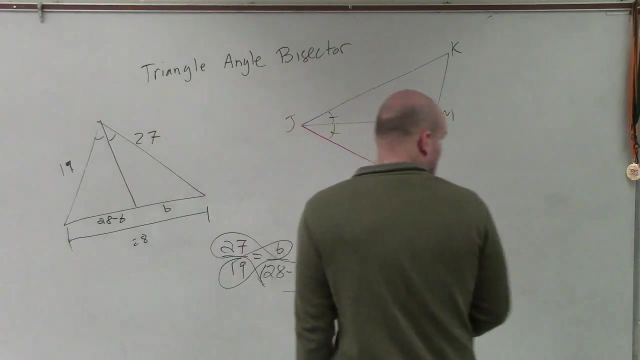 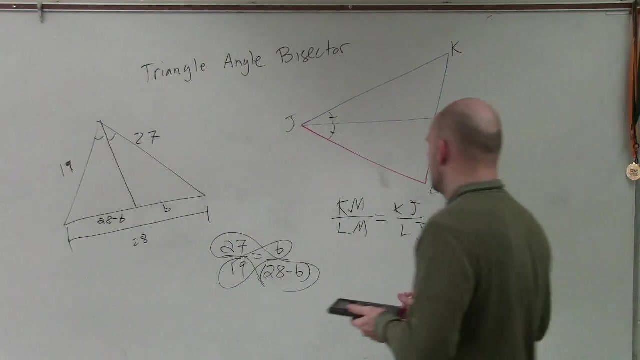 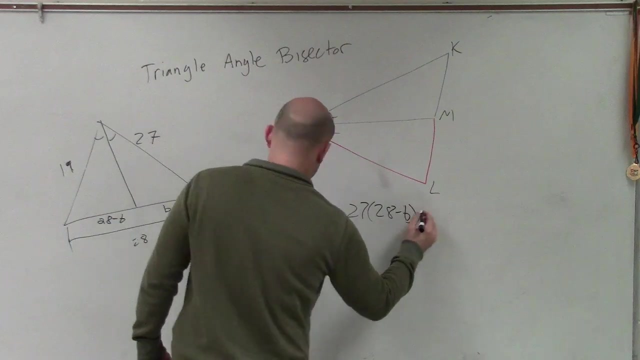 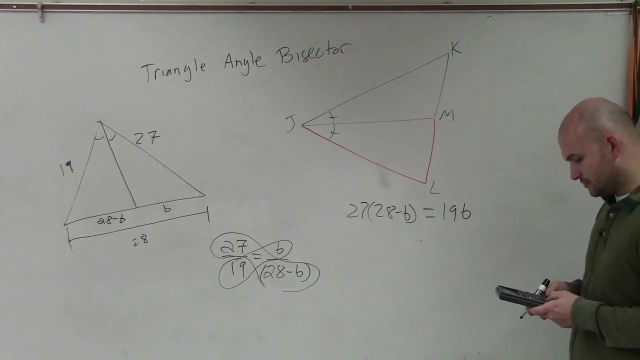 can set. Okay, Now I'll apply my cross multiplication And I will use my calculator on this one. So my calculator will say: 27 times 28 minus B equals 19 times B. So it would be 27 times 28.. So it's going to be 28 times B. 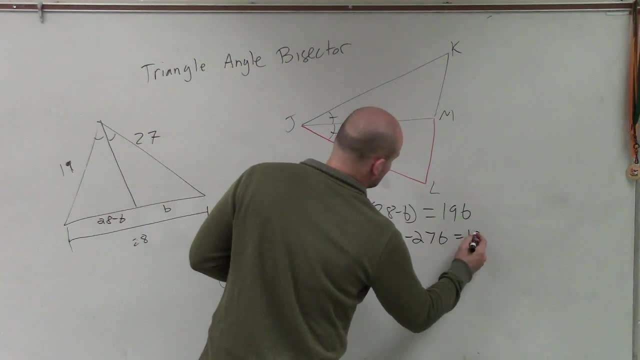 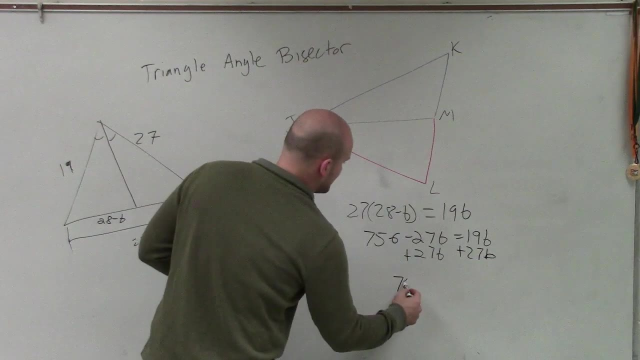 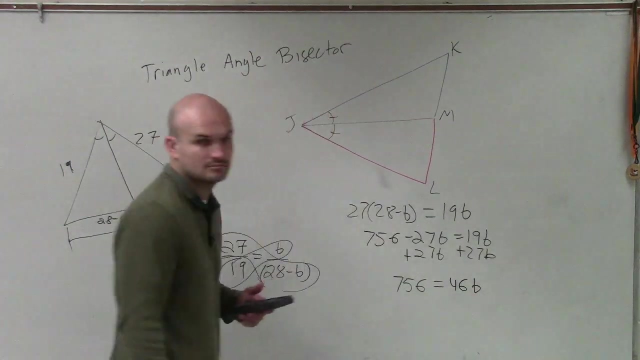 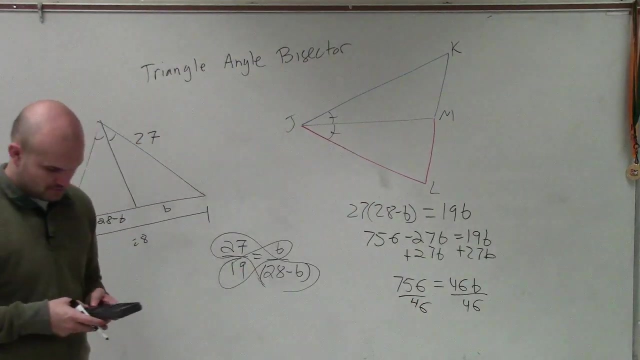 756 minus 27B equals 19B. Add 27B: 756 equals 16,, so that'd be 46B. Okay, Now I'll divide by 46.. Divide by 46.. And B equals 16.43..